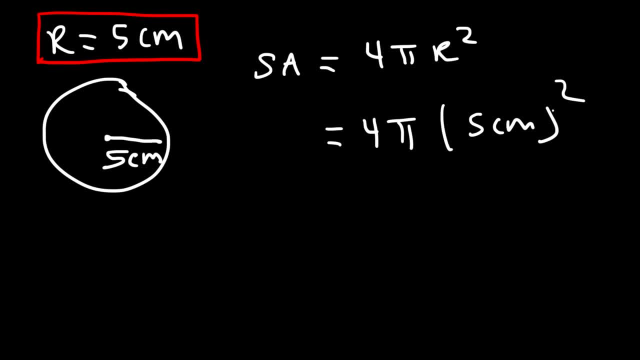 because I'm going to use the exact value of pi which is in my calculator, which is 3.14159, with some more numbers attached to it. So 4 pi times 5 squared, That's going to be basically 100 pi, which is 314.159, with some more numbers. 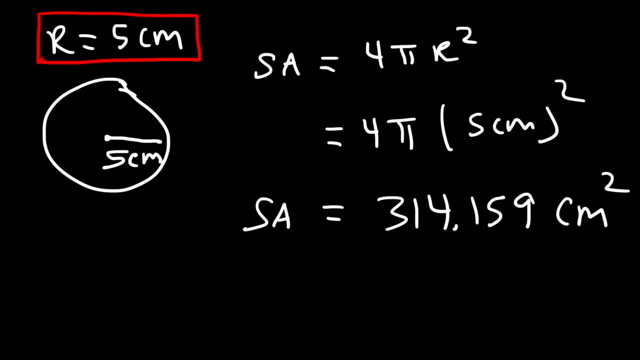 and then square centimeters. So any time you need to calculate the area of an object, your units is going to be units squared. So if this was, let's say, 5 inches, this would be inches squared, and so forth. 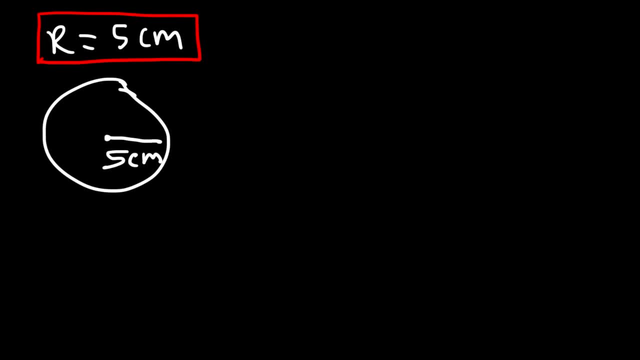 Now let's move on to the other problem. Let's calculate the volume of the sphere. So let's use this formula, And so all we need to do is we need to replace r with 5 centimeters. So what's 5 to the third power. 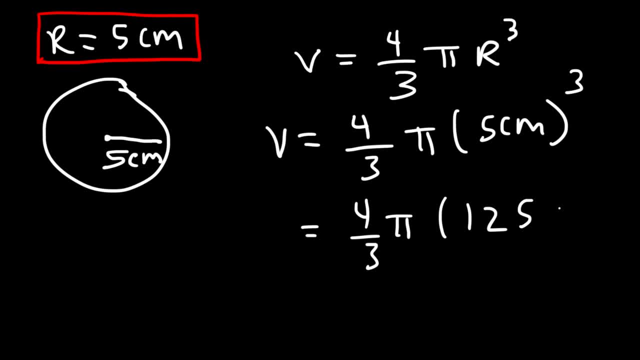 5 times. 5 times 5 is 125. And since we multiplied centimeters by centimeters by centimeters 3 times, now we have cubic centimeters. So then 125 times 4 is 500, so this is equal to 500 pi over 3 cubic centimeters. 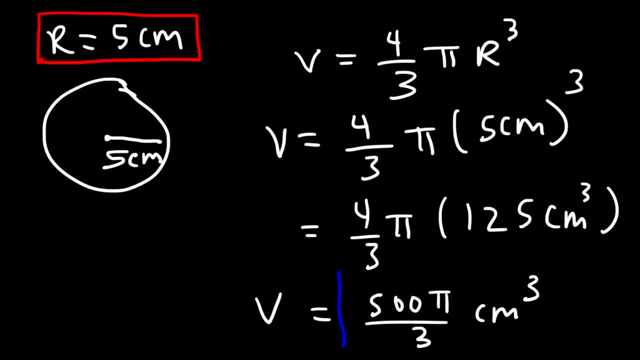 That's the exact answer for the volume of this object. but let's get the decimal value of that, So 500 times the exact value of pi over 3, so I got 523.599, if you round it cubic centimeters. 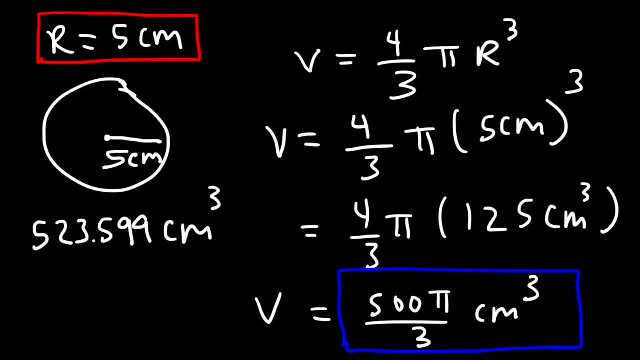 Now let's say, if you're using just 3.14 instead of the exact value of pi, The answer that you would get would be 523.3.. So it's not exactly the same, but they're still close enough. But if you use the exact value of pi, you should get this answer. 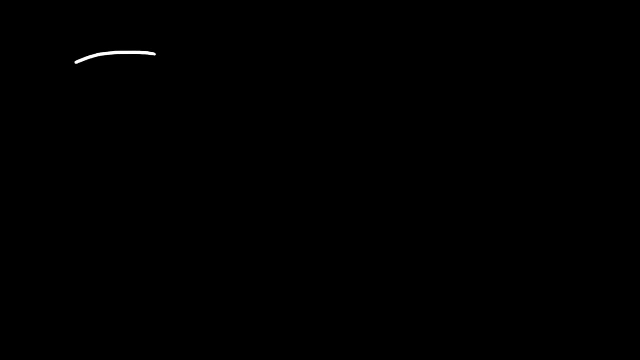 Now, the next 3D shape we're going to talk about is the cylinder, And so here is a rough sketch of the cylinder. So you need to know the volume and the surface area formulas for this type of shape. So this is the radius of the cylinder. 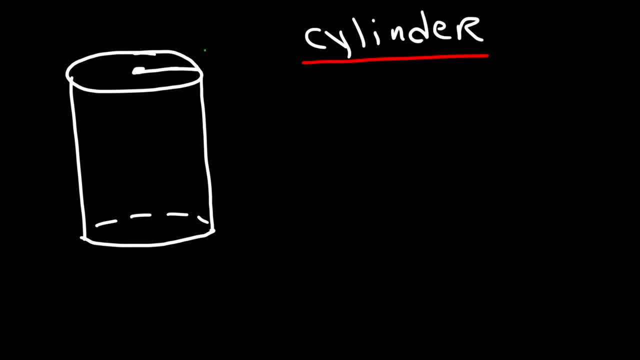 Let's put an R here. That's a terrible looking R. let's do that again. Sometimes my computer's be having issues. Now this is the height of the cylinder. Now the volume of the cylinder is the volume of the base. I mean it's the area of the base multiplied by the height. 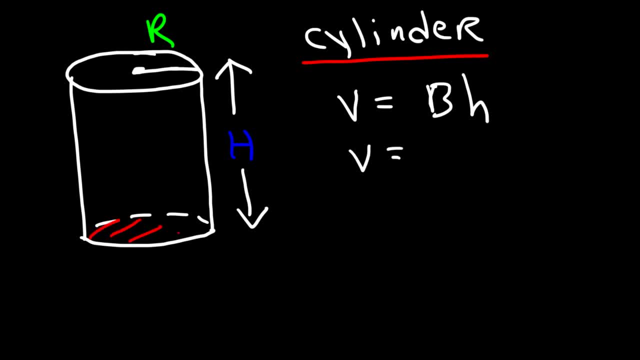 So notice that the base has the shape of a circle. And what is the area of a circle? The area of a circle is pi R squared, So that's the area of the base. And then we need to multiply that by the height. 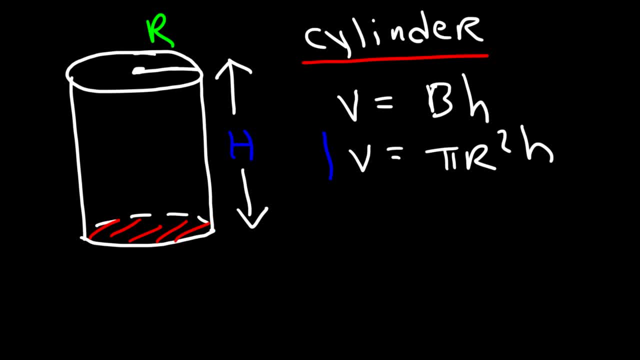 And so this gives us the area of a cylinder, which is pi R squared, times the height. It's simply the area of the base times the height of the cylinder. Now, next up, we have the surface area. The surface area of the cylinder is the area of the base plus the lateral area. 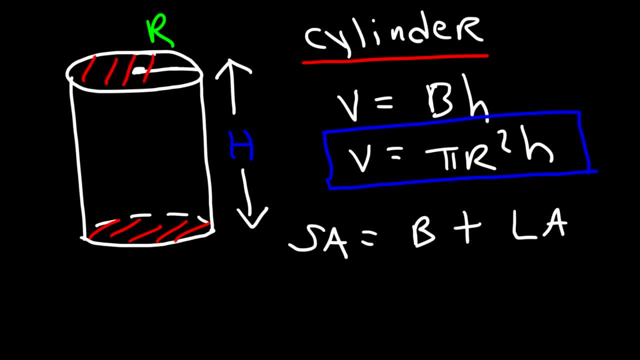 Now the area of the base is the area of a circle, but keep in mind we have a circle at the top and at the bottom, So it's going to be pi R squared, but times 2.. Now what about the lateral area? 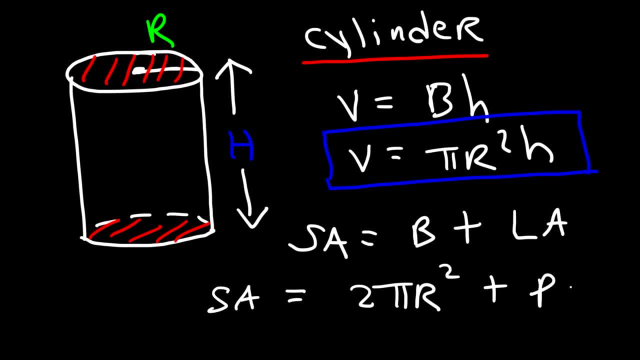 The lateral area is the perimeter multiplied by the length, But it's going to be the perimeter of the base. So what is the perimeter of a circle? The perimeter of a circle is the circumference of a circle, And the circumference of a circle is 2 pi R. 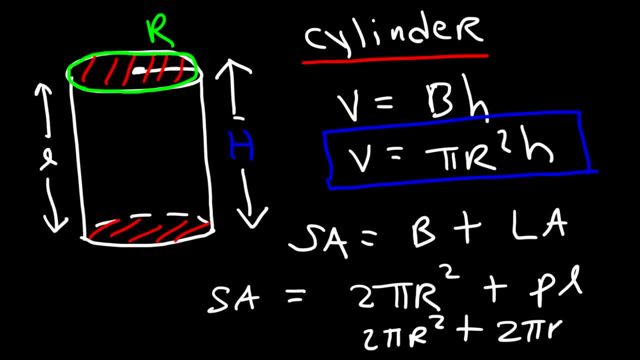 Now, the length of the cylinder is the same as the height, So that's how we can get area of the cylinder. So it's 2 pi r squared plus 2 pi rh, where r is the radius of the cylinder, or the circle in the cylinder, and h is the height of the 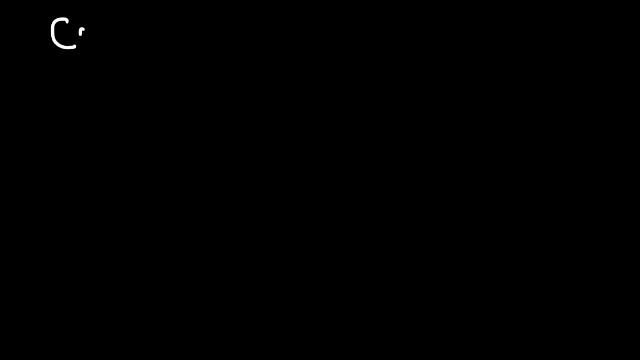 cylinder. Now, the next shape we're going to talk about is the cone, So here's one way in which you can draw the cone, And so here we have the radius of the cone, and this is the height of the cone. So that's h, and notice that we have a. 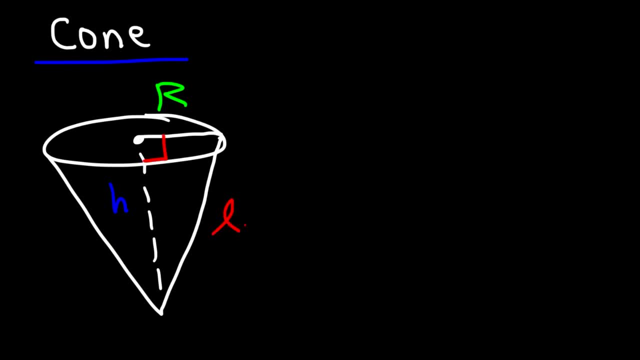 right triangle on the inside, L is known as the slant height. So what are the formulas for the volume of a cone and the surface area of a cone? The volume is very similar to the volume of a cylinder. Imagine if you drew a cylinder. 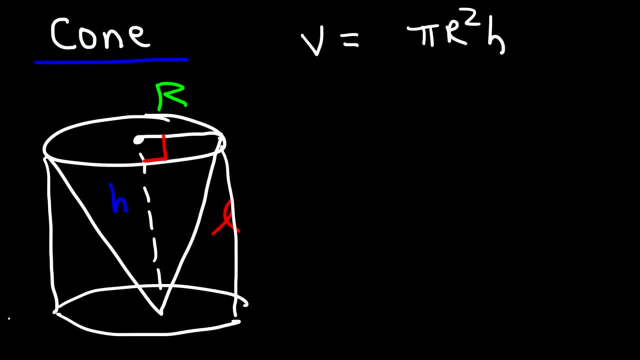 So imagine if you drew a cylinder. But it turns out that the volume of a cone is one-third that of a cylinder, So it's just one-third pi r squared times the height. Now what about the surface area? The surface area of the cone is going to be the area of the base plus. 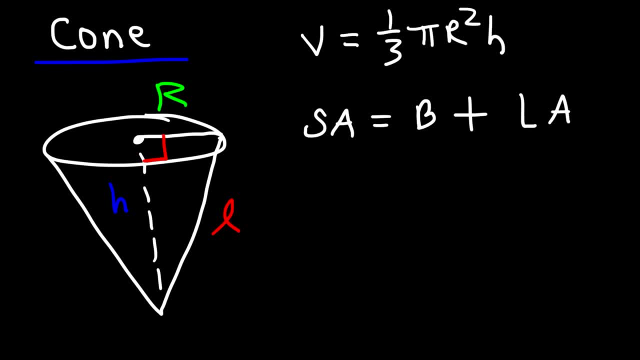 the lateral area, And we know the area of the base is going to be the area of the circle. That's the base. So the area of the circle is pi? r squared times the slant height. Now, what about the lateral area? It turns out that for this shape, 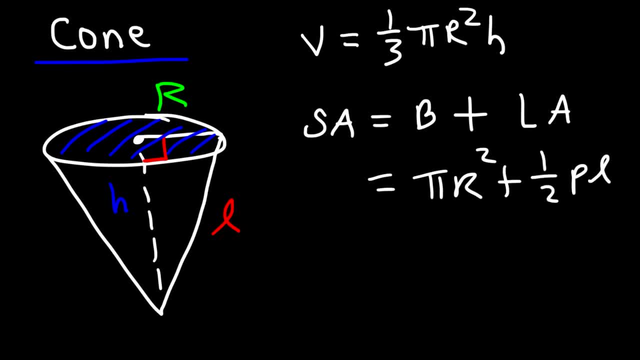 it's one-half the perimeter times the slant height, instead of just PL. Now the perimeter is going to be like last time: It's going to be the circumference of the circle, which is 2 pi r. So we have one-half 2 pi r and then times the 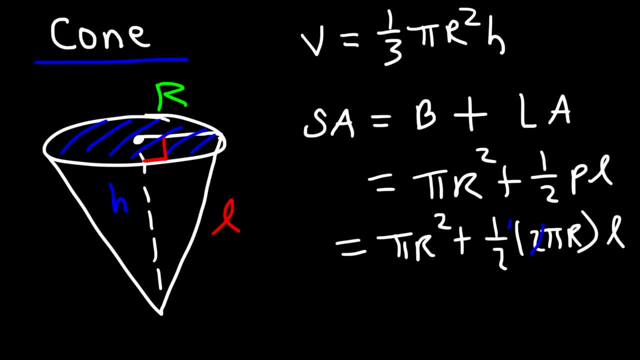 slant height. So we could cancel one-half in 2, because half times 2 is 1.. And so we get this formula: for the surface area of a cone It's pi r squared plus pi r L, where L is the slant. 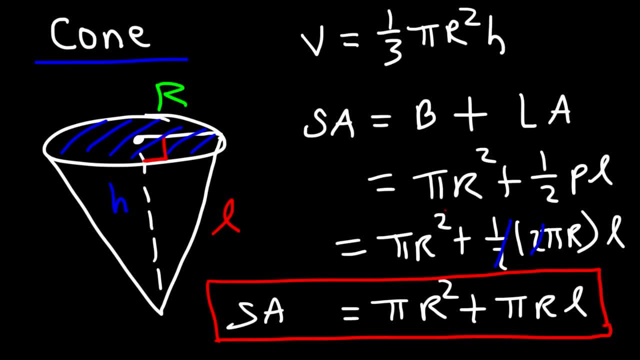 height, as we mentioned before. So how do we go about finding the value of L? To find the value of L, you need to use the Pythagorean theorem. Notice that we have a right triangle with those three sides. So, based on the Pythagorean theorem, c squared is equal to a squared plus b. 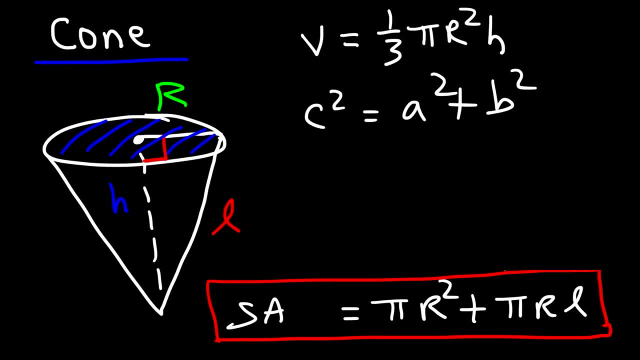 squared, In this case c is the length of the hypotenuse, which is going to be the slant height. So L squared is equal to r squared plus h squared. So therefore, L, the slant height, can be found using this equation. So if you need to calculate the 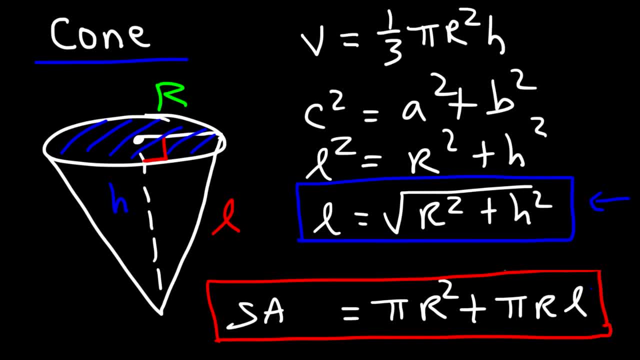 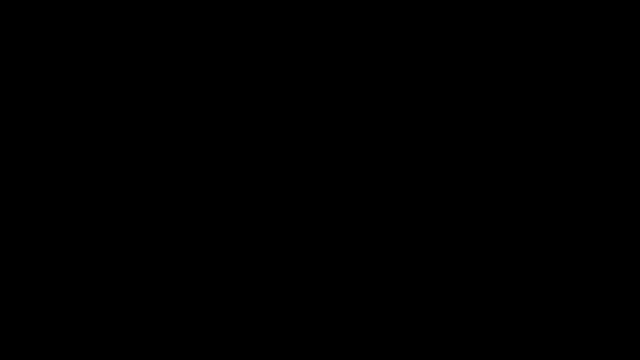 surface area. find the slant height and then use that with the radius to find the surface area of the cone. And then here's the other formula: you need the volume of a cone Now. the next shape I want to talk about is the rectangular prism. Let's see if I can draw a decent shape for it. So 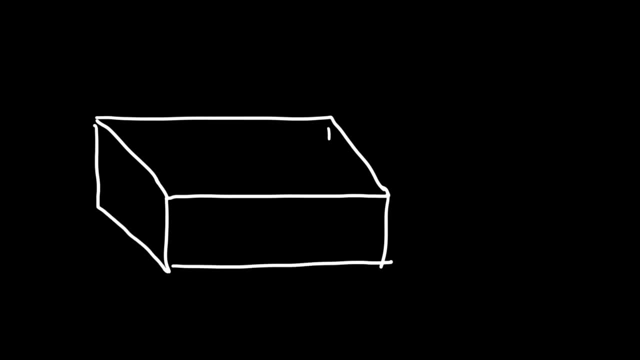 basically, it looks like a box And here it is. So let's call this the length, the width and the height. So what is the volume of the rectangular prism? The volume of any prism is the area of the base times the height. So let's review this as the base. 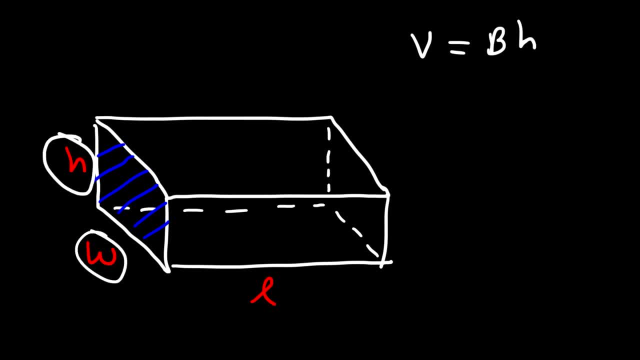 The area of the base is basically the height times width, based on what we drew, And then the height of the prism is the same as the length, so we can replace h with L, And that's going to give us this equation: The volume of a rectangular. 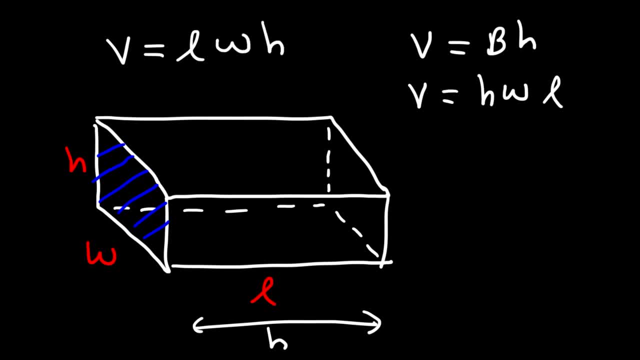 prism is the length times the width times the height, And I prefer to remember this formula in this form. It's just easier. Now the surface area of a rectangular prism. I'm just going to give you the formula: It's 2LW plus 2WH plus 2LH. 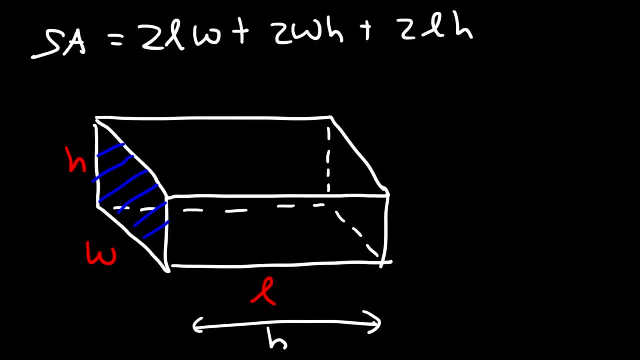 Now, if you want to know how to get it, if you find the area of, let's say, this side and this side, it's going to be W times H, but there's two of them, so you have 2WH. 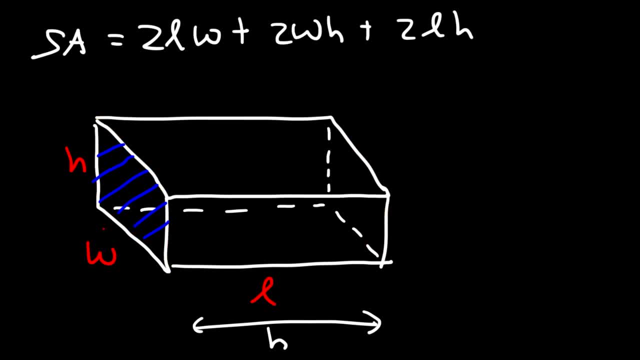 So that's for the left side and the right side. Now, if you calculate the area of the top part of the prism and the bottom part, notice that it's L times W, so it's going to be 2LW. And then, if you take the area of the face in the front, 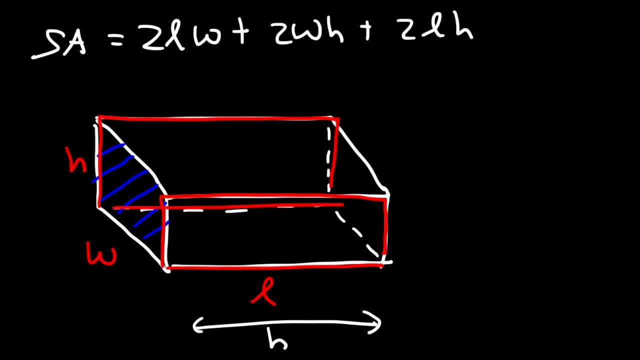 and the face that's in the back, it's going to be L times H, so you get 2LH. So you've got to find the area of each of those six faces and then add it up, Or you could simply use this formula: 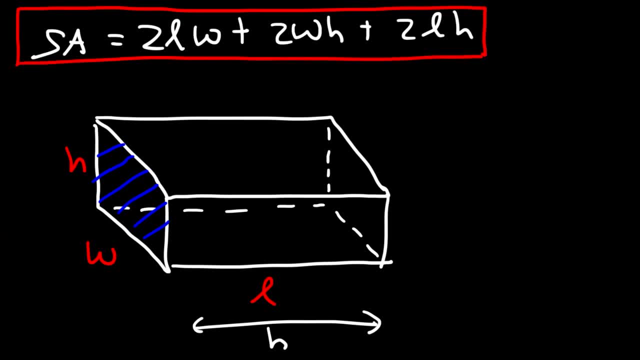 So that's how you can calculate the surface area of a rectangular prism. Now let's call this point A and point B. So what is the distance between point A and B? How can we find the length? How can we find the length of the diagonal of a rectangular prism? 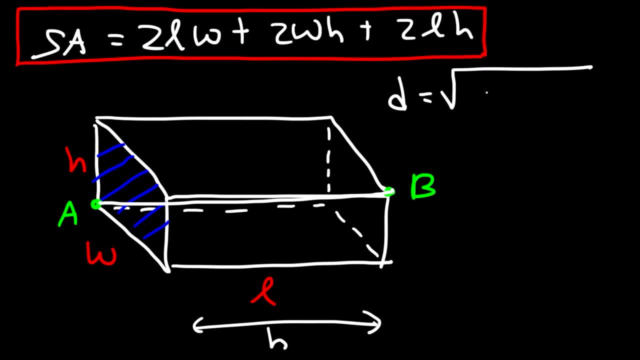 The diagonal length. it turns out it's the square root of W squared plus H squared plus L squared. So in another video where I talked about rectangular prisms, I explained how you can get that formula, but I'm not going to do it in this video. 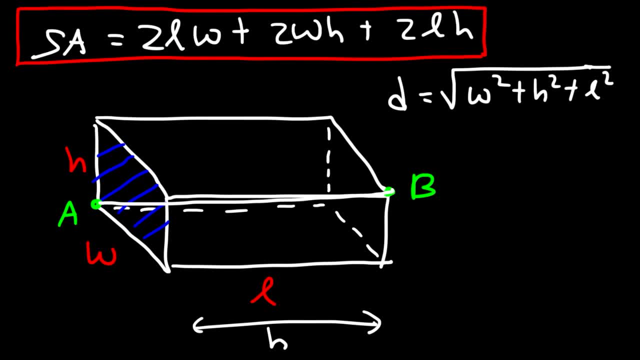 But if you look up another video I have on YouTube like volume, surface area and diagonal length of a rectangular prism, you could find it. If you want more, you can find more information on that, But just in case you need to. 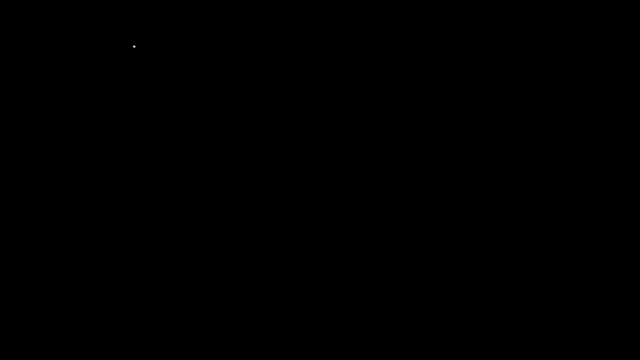 that's the formula to find the diagonal length of a prism. Now, the last thing we're going to talk about is the cube, And so first let's draw a picture, And so here's a rough sketch of a cube, And what you need to know about a cube is that 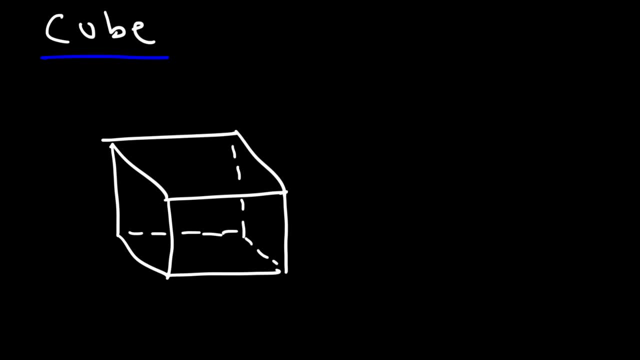 all sides are equal. I know my picture looks terrible, but we'll work with it. So we can say that that each side is X. Now we know that the volume of a rectangular prism is the length times the width times the height. 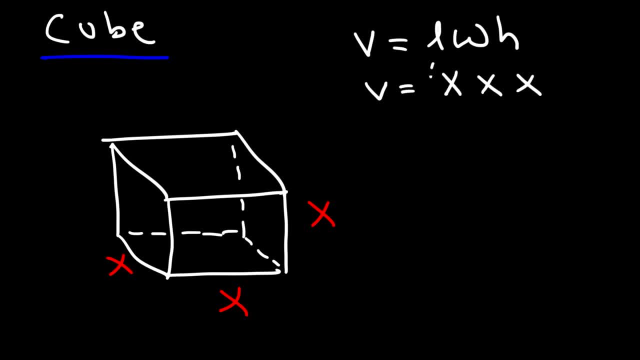 For a cube it's going to be X times X times X, which is going to be X cubed or side cubed. So that's the volume of a cube. Now, the surface area of a cube is going to be the area of all six faces. 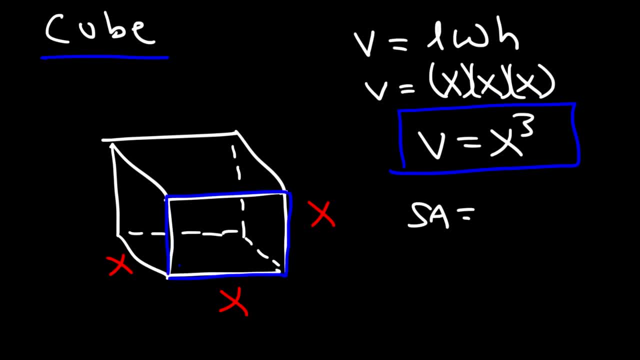 The area of just one face is X times X or X squared. Since we have six of them, it's going to be six X squared. Now, the last thing we need to talk about is the diagonal length of a cube, So the distance between points A and B. 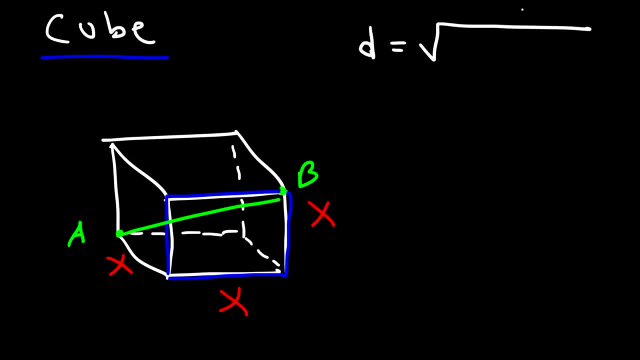 Now we're going to start with this formula, And that is the diagonal length for a rectangular prism: W, L and H. they're all equal to X when dealing with a cube. So 1X squared plus 1X squared plus 1X squared. 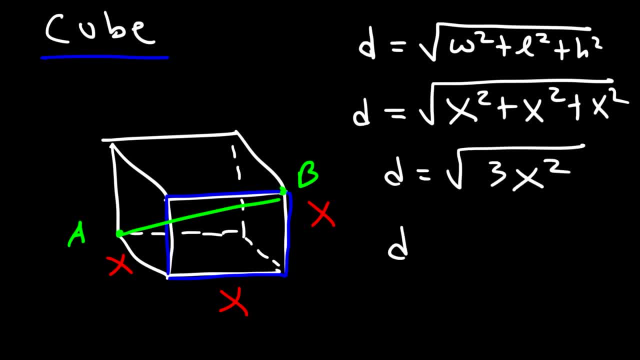 is going to be 3X squared, And the square root of 3X squared is the same as the square root of 3 times the square root of X squared, And the square root of X squared has the same magnitude as X, So the diagonal length is going to be the square root of 3 times X.